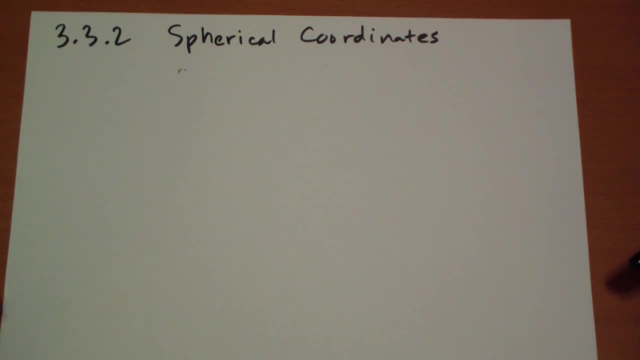 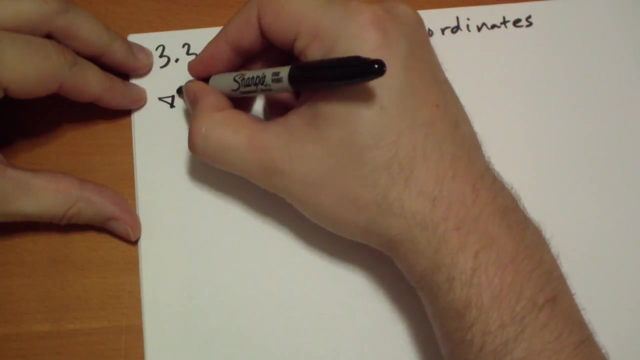 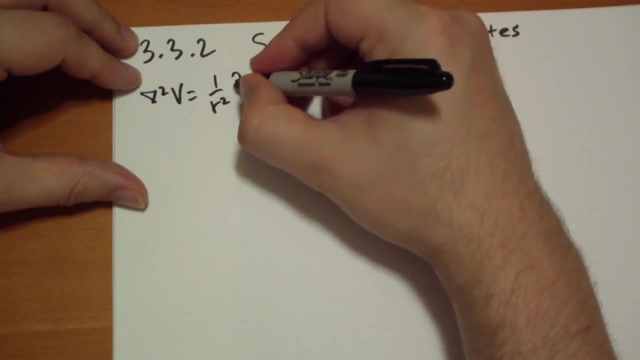 When you tackle spherical coordinates, it's not impossible, and just you know, take it piecemeal, bit by bit. The Laplacian and spherical coordinates is not anything like the Laplacian and Cartesian coordinates. So this is what it is. Let me write it out for you. You can find this on the inside cover of your book too. 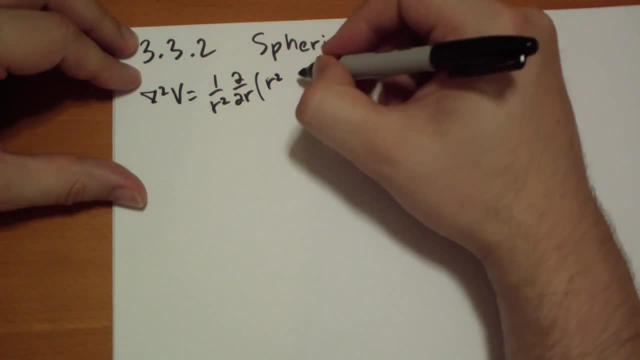 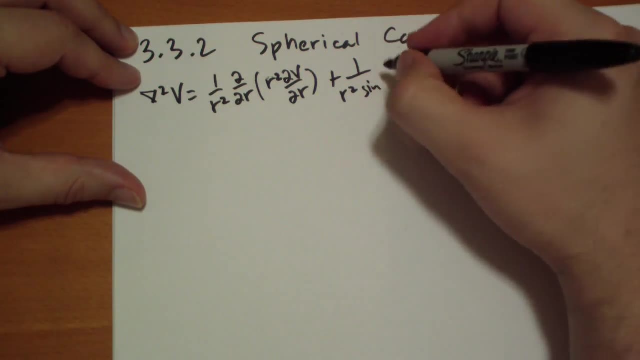 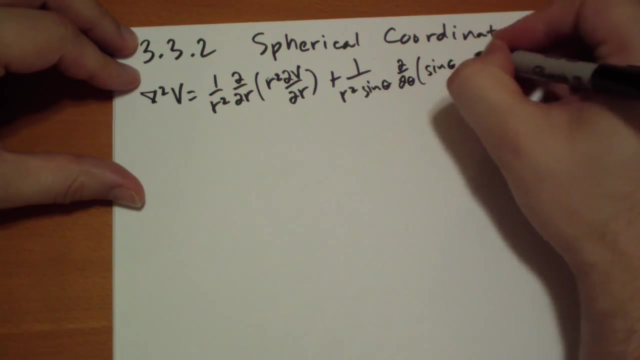 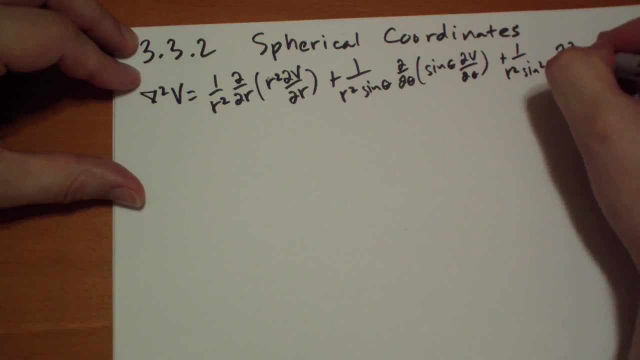 So dv by dr plus 1 over r squared sine theta d by d theta. of sine theta dv by d theta- Am I going to fit it? Probably 1 over r squared sine squared. theta d by d theta. d squared by d phi, squared. 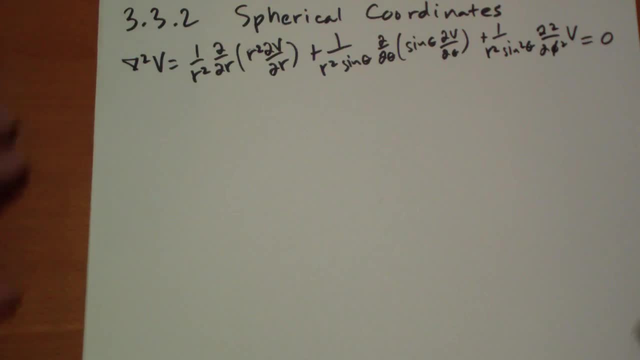 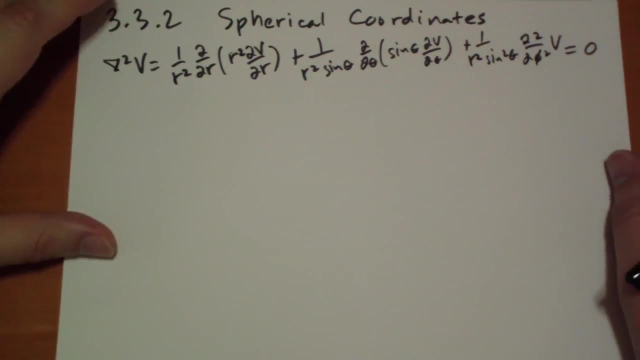 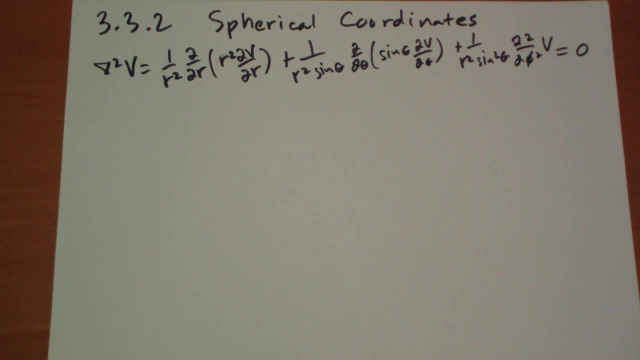 If you memorize that, you probably deserve a pat on the back. Once again, there's three components. Each of them have a double integral. Sometimes there's this funky thing that you have to put in the middle. So now what? Hopefully the focus isn't too bad. 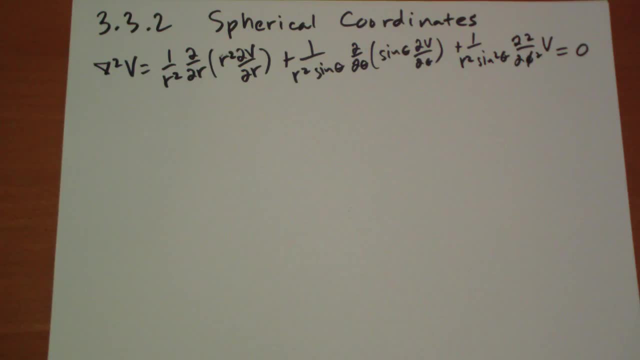 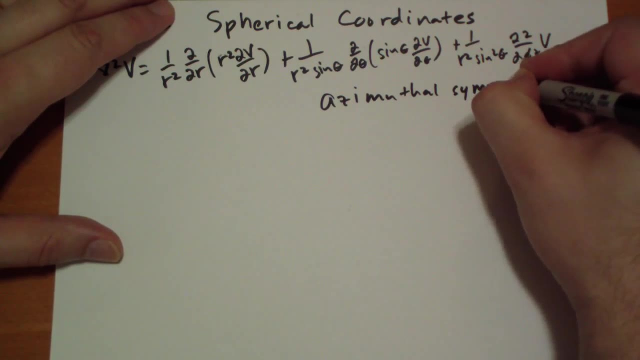 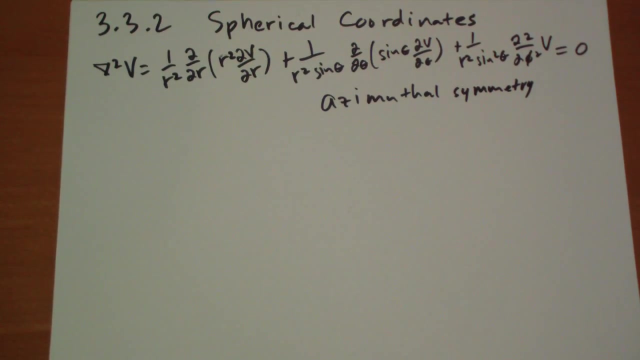 Well, we're going to assume azimuthal symmetry, And the reason why is because we don't want to kill ourselves. The math exists to solve these things, I believe. I haven't looked at it for a while and unless you're paying me a lot of money, I'm not going to solve it. 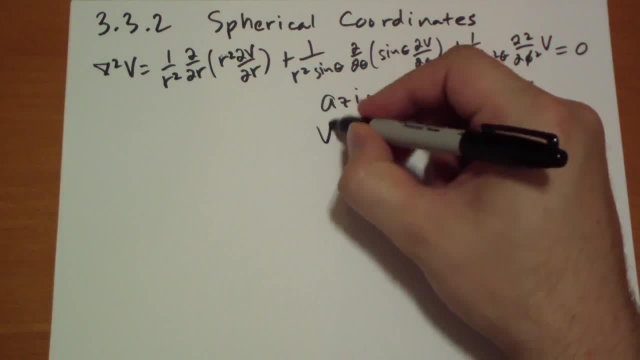 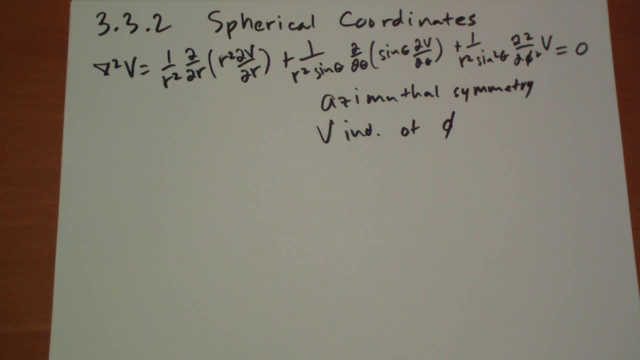 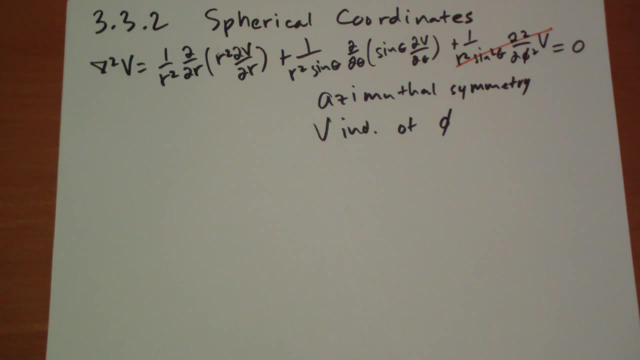 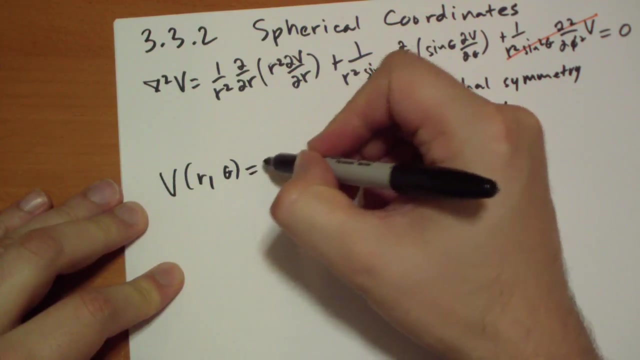 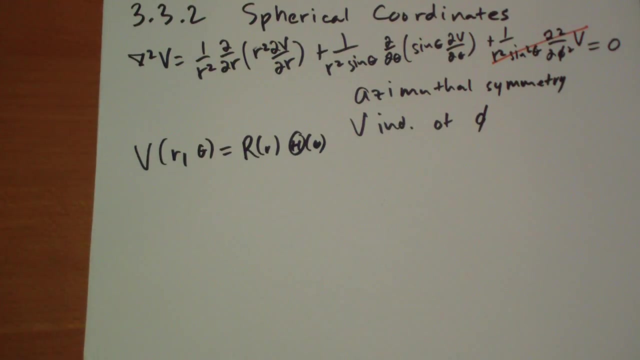 So that means v independent of phi, So we can just drop this phi term when azimuthal symmetry is in effect. Okay, And we're going to look for solutions that look like this: That's that theta. It looks like chubby cheeks, but that's a big capital theta. 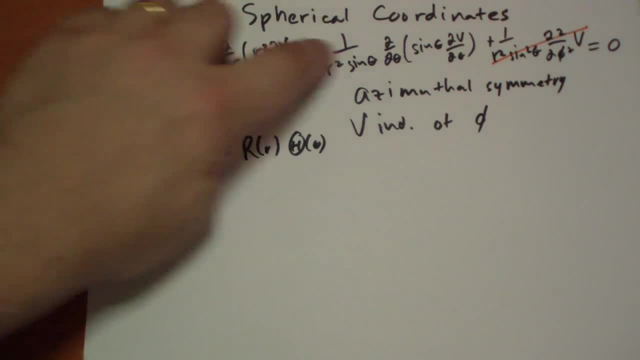 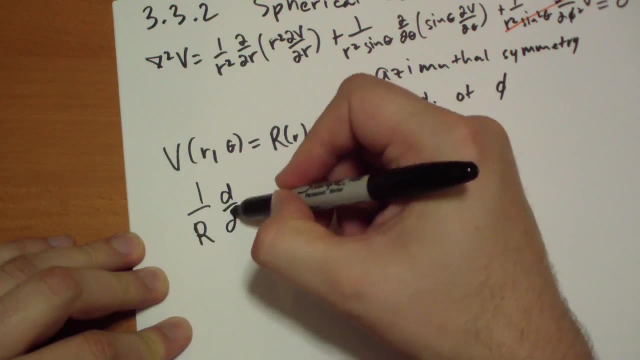 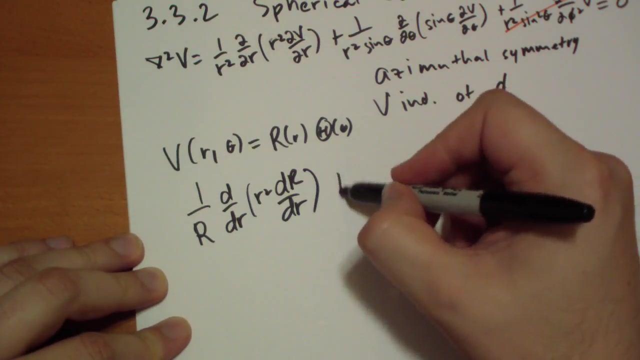 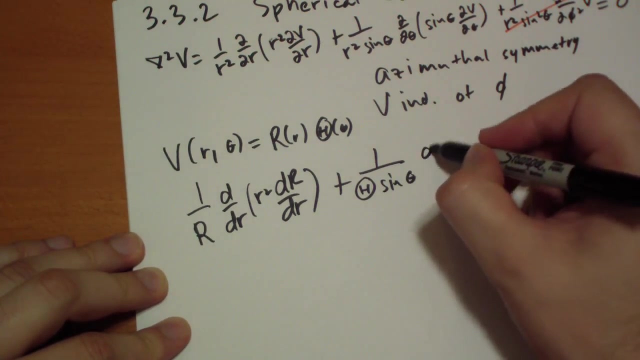 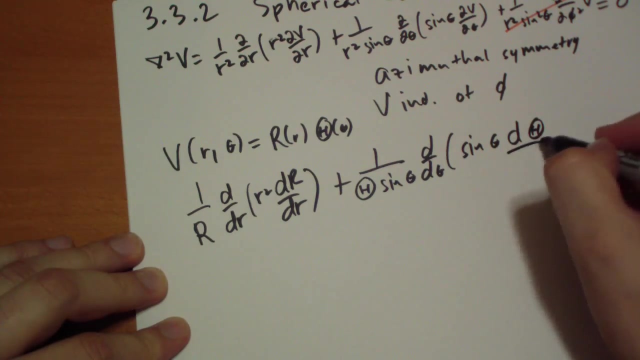 And when we plug this in to this differential, we get 1 over r. d by dr of r, squared dr by dr, plus 1 over capital theta sine lowercase theta. d by d theta sine theta d capital theta over d theta. 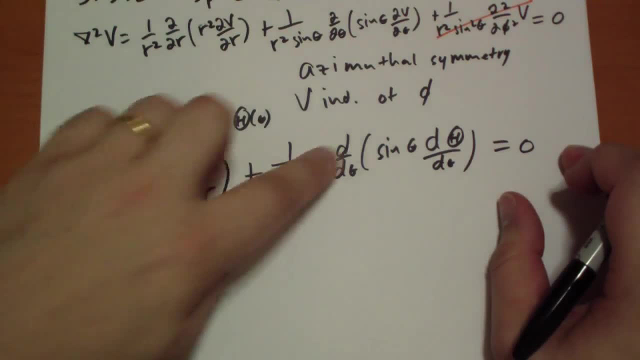 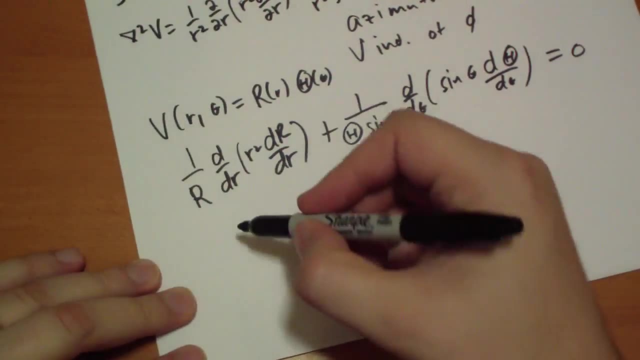 That has to equal 0.. And once again, there's only r terms here and there's only theta terms here, so these have to be constant, And the thing that he uses is he says: let's set this equal to l times l plus 1.. 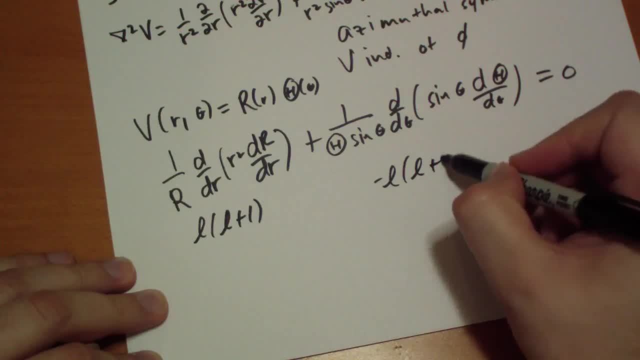 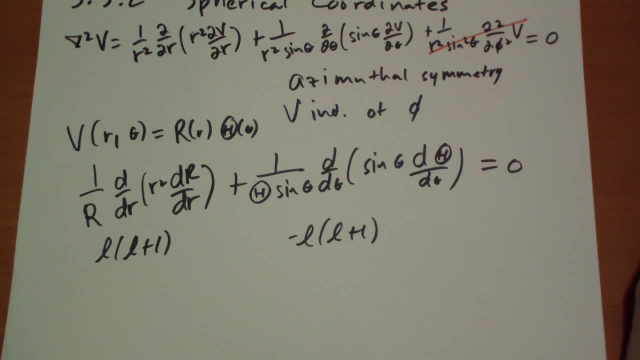 And let's set this equal to minus l times l plus 1.. And unless you've done these problems before or seen someone do them, I don't know how you're going to come up with that. So kudos to the first person that figured this out. 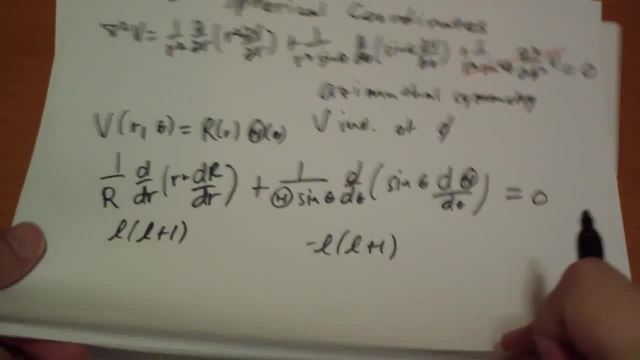 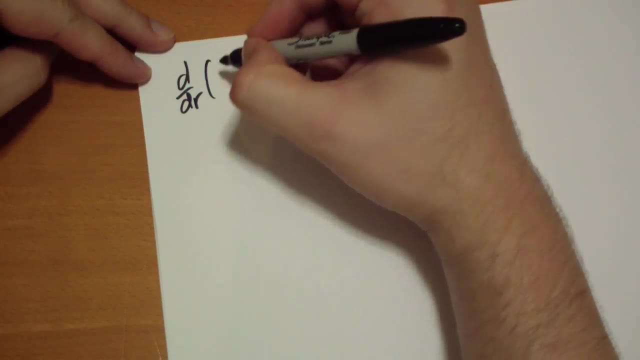 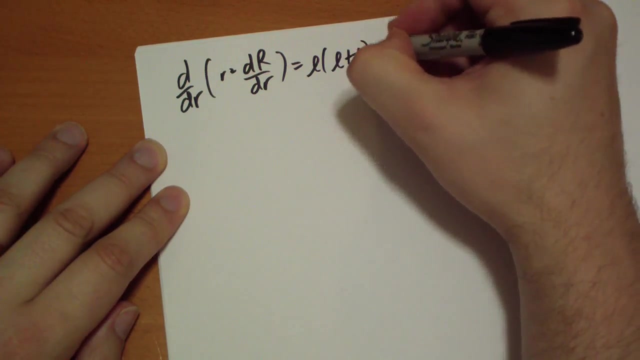 Okay, So for the r term we just multiply both sides by r, so we get d by dr of r squared d. capital r by dr equals to l times l plus 1 of capital r And the general solution to this. 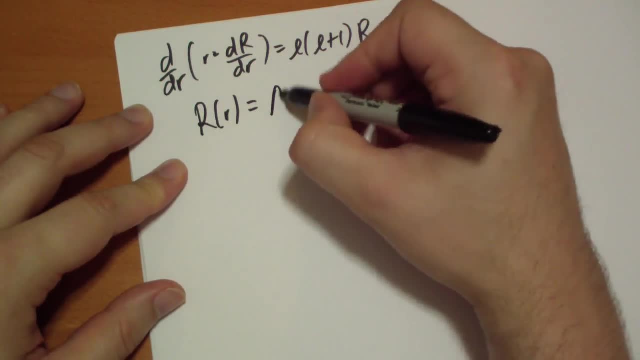 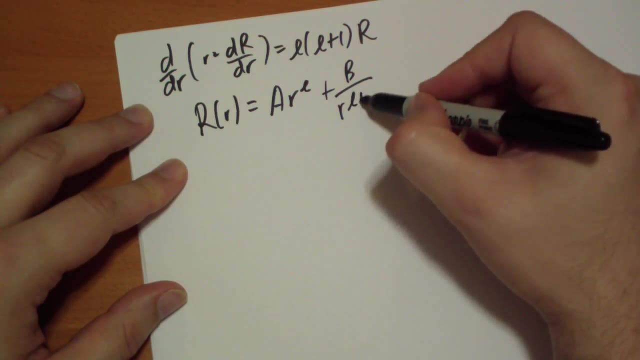 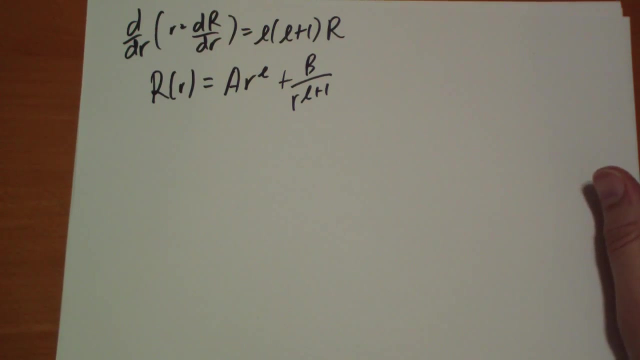 is that r of r is equal to some constant times, r to the l plus b, another constant over r to the l plus 1.. You take this and apply this derivative. you get that For the theta term. so we have: 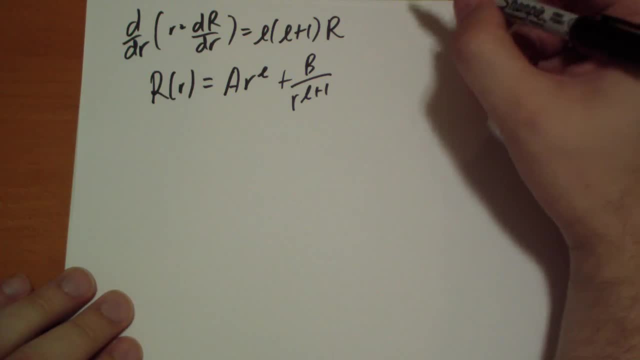 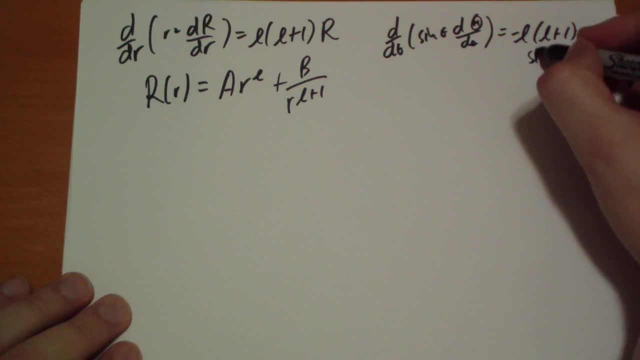 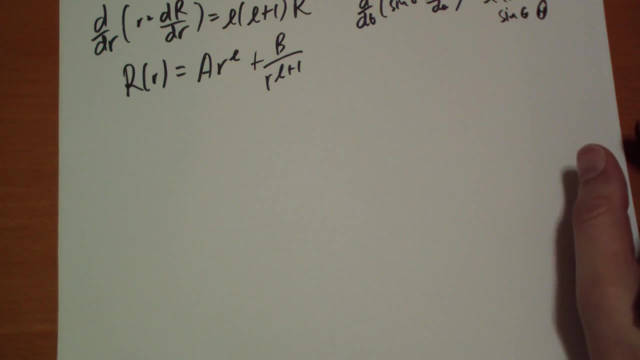 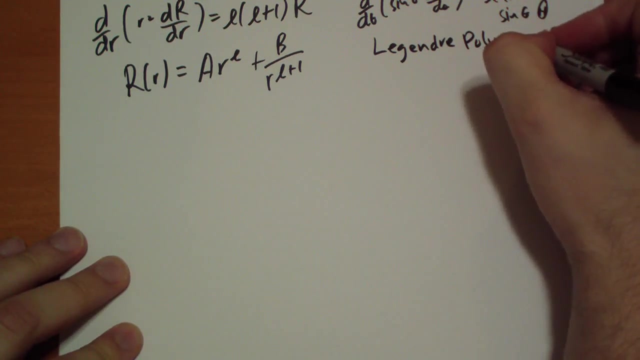 How did that work? Oh yeah, So we get d by d theta, of sine theta, d capital theta by d theta is equal to minus l times l plus 1 sine theta and capital theta. Okay, And this has the solution of Legendre polynomials. 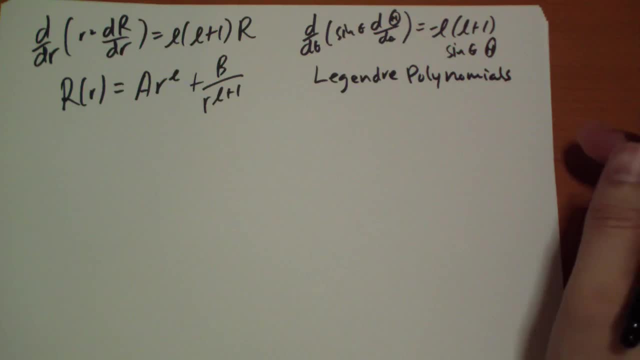 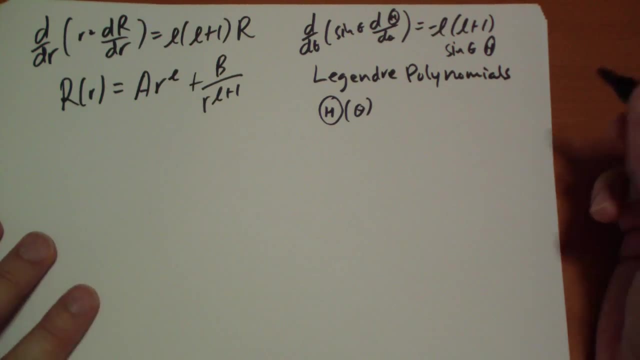 Okay, Again, don't freak out. This is not that difficult. Besides, I don't think you're going to be asked to be doing too much with these. so Of cos theta And the p? l, this is the Rodriguez formula. 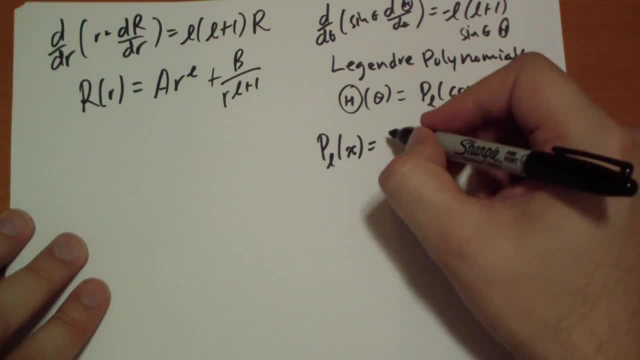 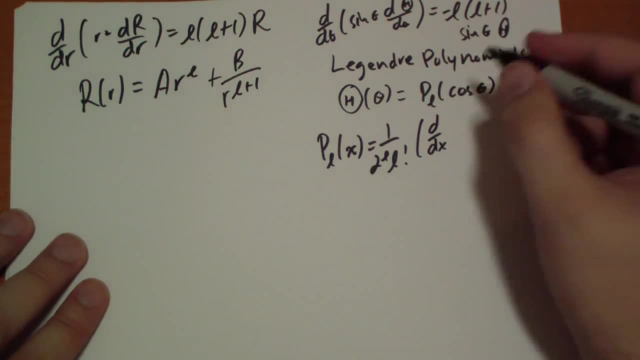 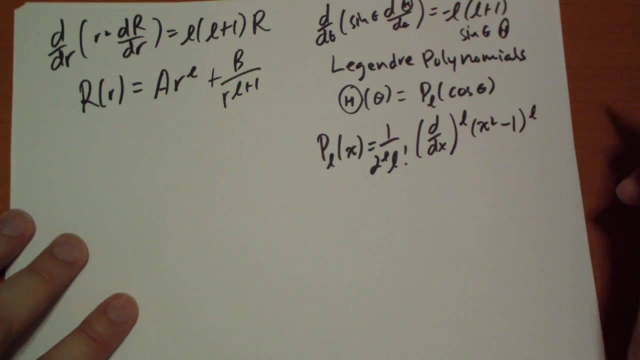 so p? l of x is equal to 1 over 2 to the l- l factorial times. You didn't think that was all, did you? d by dx, the lth derivative of x, squared minus 1 to the l. 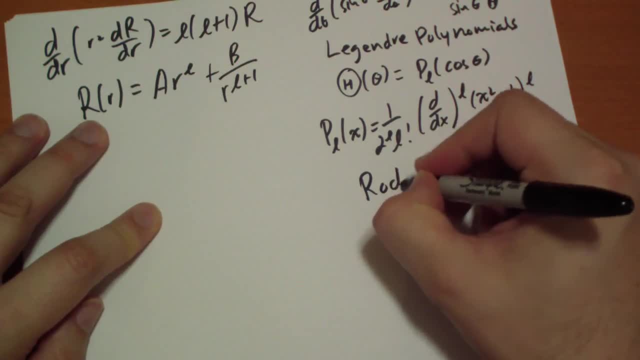 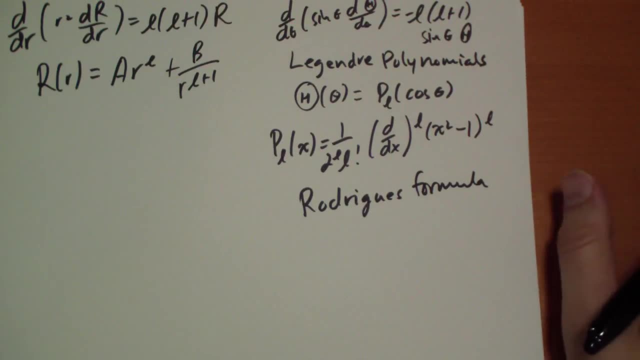 This is called the Rodriguez formula- Rodriguez, Okay, And I encourage you to calculate the first few yourself, just so you know what they look like In practice. if you're given simple enough problems, you won't have to know more than a couple. 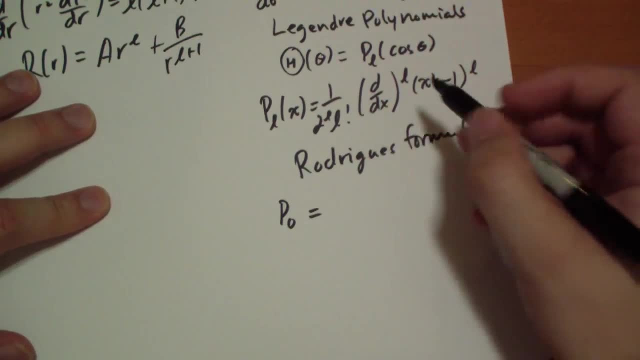 Let's just write out a couple. So p 0 is equal to- let's see 1 over 2 to the 0,, which is 1,. 0 factorial is 1, the 0th derivative of x squared minus 1 to the 0.. 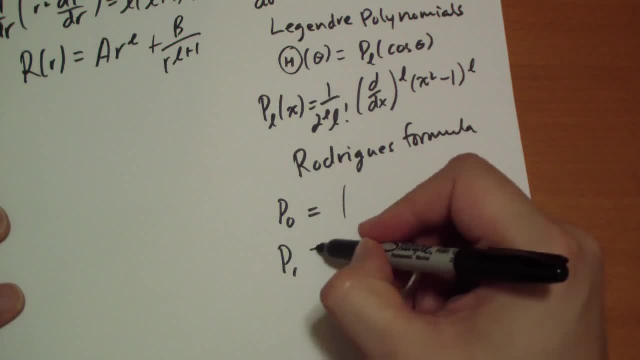 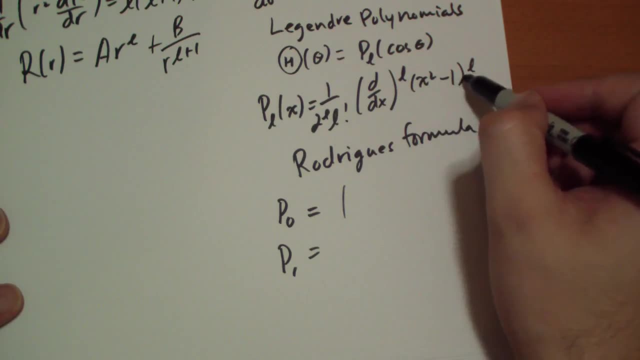 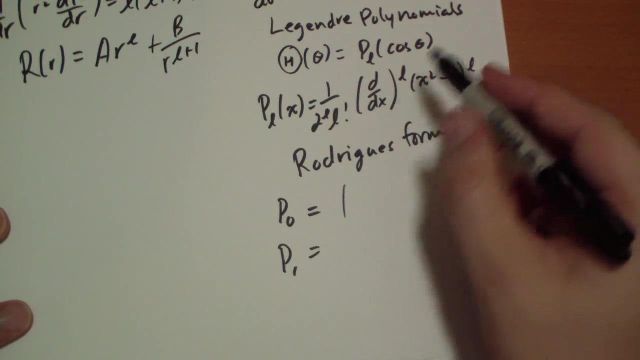 So it's just 1.. p 1 is 1 over 2 to the first. power times 1 times the first derivative of x squared minus 1 to the 1.. So that's just 1. half of x squared. derivative of x squared is x. 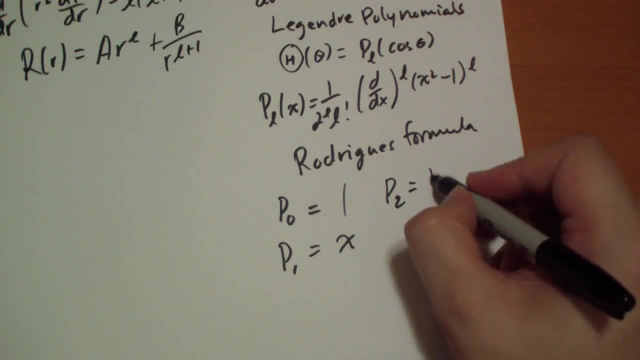 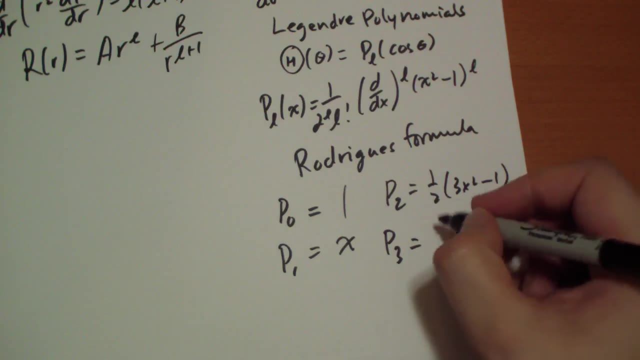 p 2 is a little bit more complicated. You're going to end up with 1, half of 3x squared minus 1.. And p 3 is, as you might imagine is going to be something with an x cubed term. 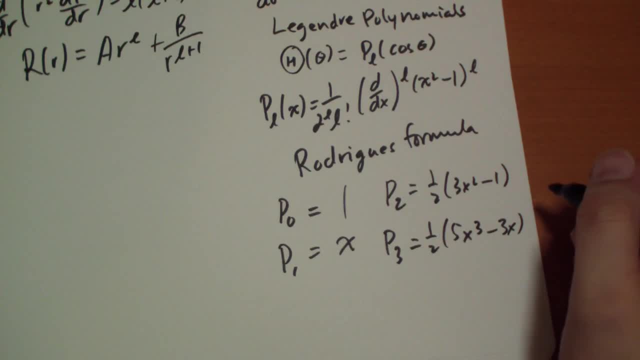 This one actually is minus 3x And from there it grows more complicated And you can look in the book and you can have some fun with this if you want. But the important thing to notice is that p 0 has no x's in it. 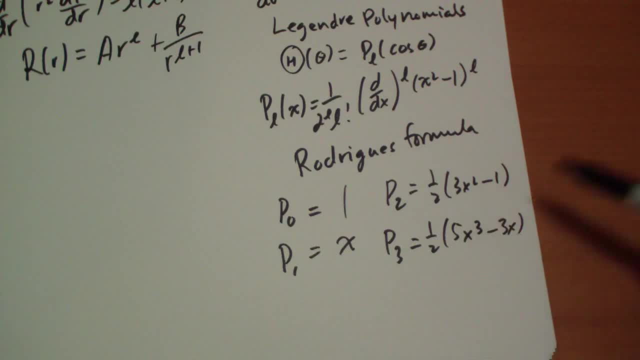 p 1 has 1x, p 2 has x squared, p 3 has an x cubed term. So these are polynomials. The obviously this only works when you have l greater than 0 and l is an integer. 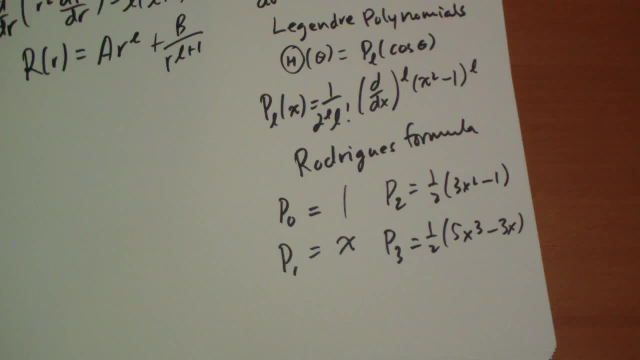 I'm not excited about finding the factorial of a fraction, so If you were to try to calculate the like 0th Legendre polynomial, oh no, here. let me put this differently: p? l of 1 is 1,.